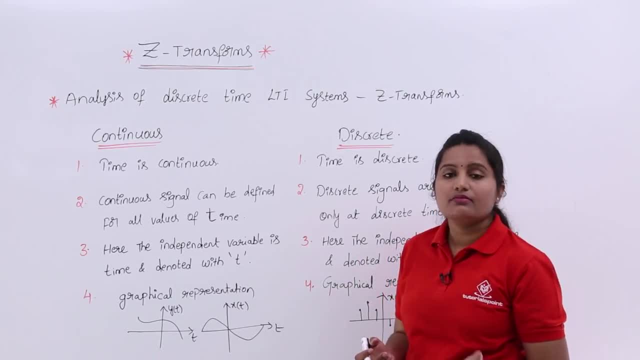 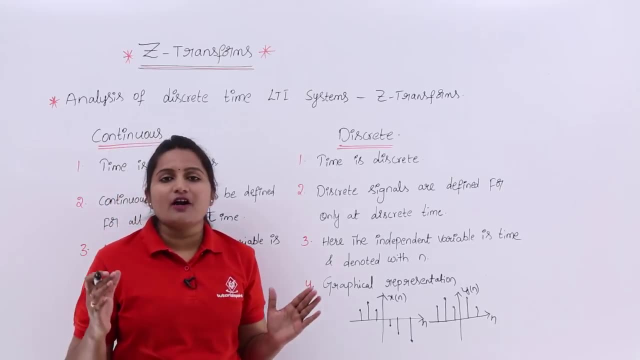 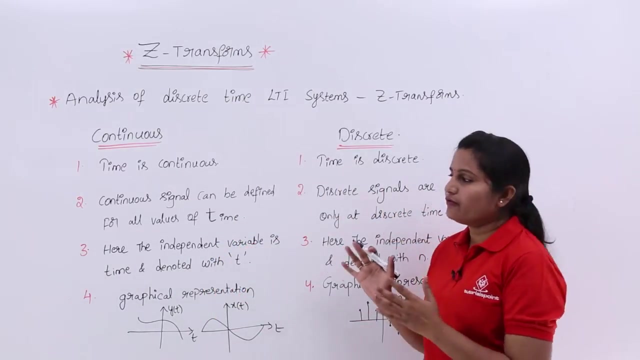 get frequency domain of the discrete time signals by using jet transform. also Before getting into jet transform concept here I want to discuss about the discrete time Fourier transform. Here I want to consider the fundamental difference of continuous time and discrete time signals. Here I listed very important 4 points which gives the fundamental difference. 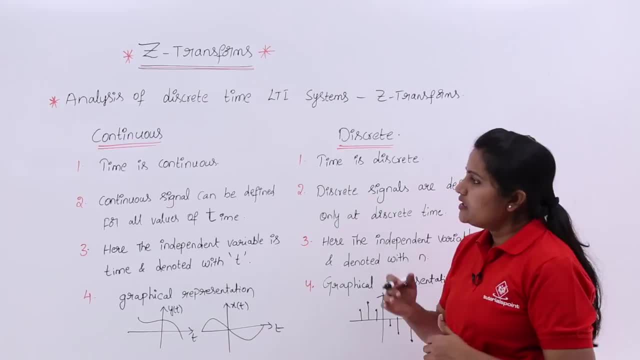 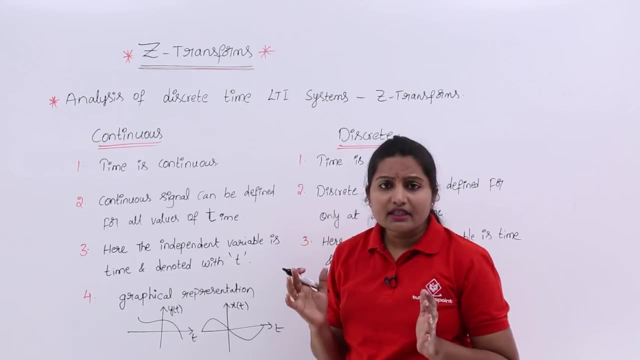 between continuous and discrete time systems. So coming to continuous time system, or signal, time is continuous here. Whatever the time is there, that is continuous, it is not going to cut anywhere. So if 1 is the time, 1.1 is there, 1.2 is there, 1.001 is there, 1.002 is there? like, 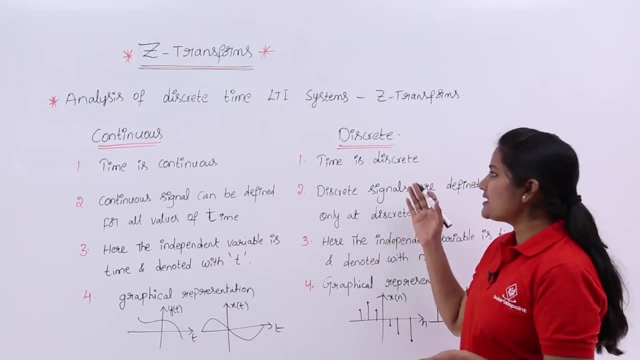 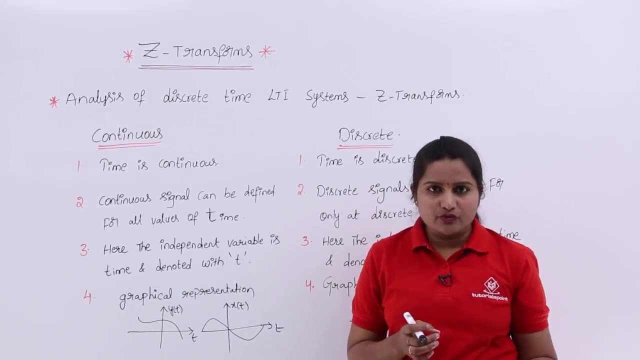 that here time is continuous, whereas in discrete time system time is discrete, not continuous. That means if you are having your value at one time period, again you will get another sample or value of the signal at 2,, 3, 4. only at integer values you are going to have your. 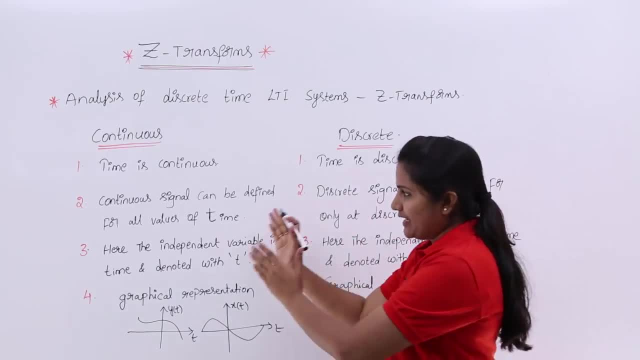 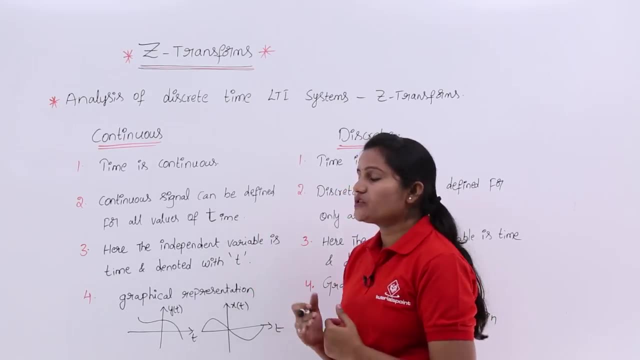 your signal value. So now coming to the second important point about continuous. Continuous signal can be defined for all values of time, For example. if you want to define any signal, for example, here you can see, these are the graphical representation of the signals. So 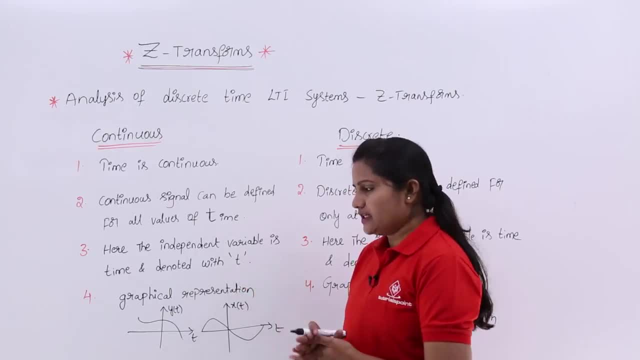 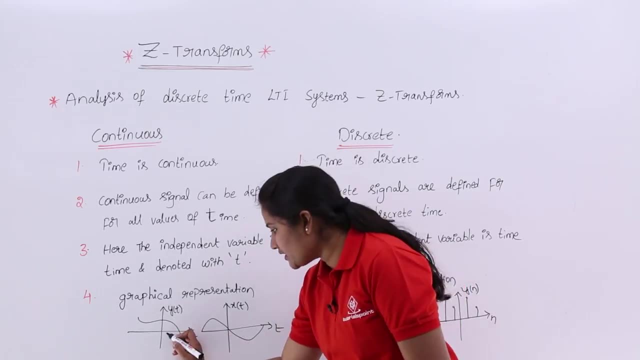 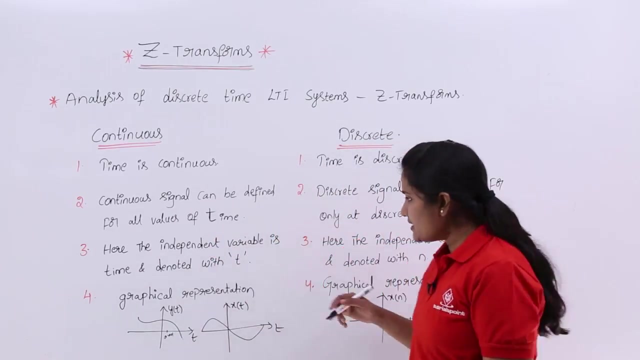 here, when you are defining continuous signal, it we can define it all intervals of time. For example, if this signal is given, they are asking: what is the signal value at 0.001.. You can trace that value, Whereas in discrete time signal, discrete signals are defined for. 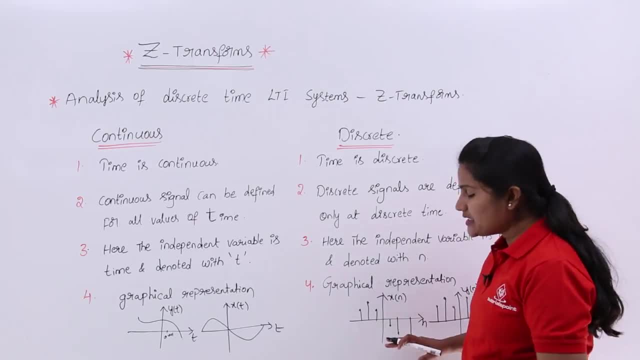 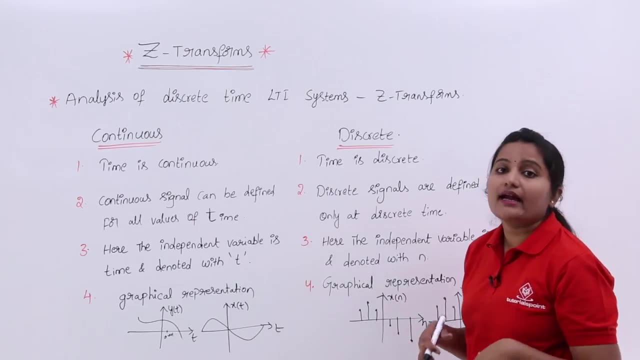 only at discrete intervals of time. So as discrete signals are defined only at a discrete values of time, we can't trace the value of signal at continuous intervals If this signal is given, as this is a discrete signal. If they are asking: what is the value of 0.001? when t is equivalent to 0.001, what is the signal? 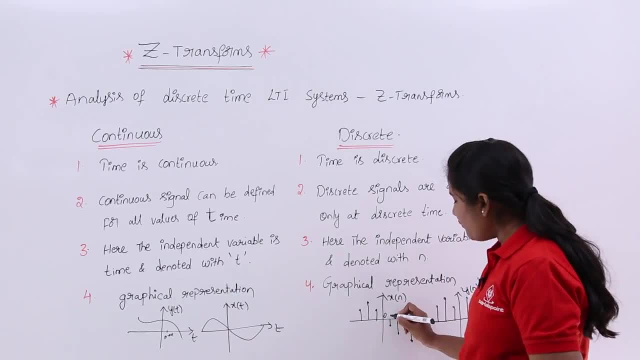 value means we can't trace Why, because they will provide the samples or signal values at discrete intervals of time: 1, 2, 3 or minus 1, minus 2, like this. So for discrete signals, these discrete signals are defined only at discrete intervals of time. Coming to third. 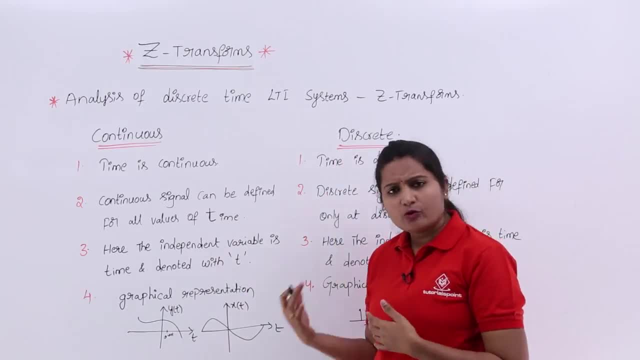 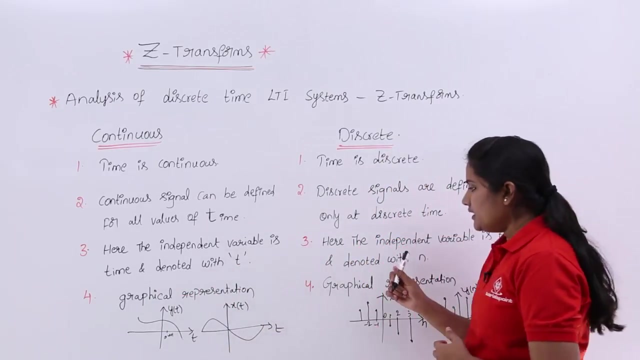 point. here the independent variable is time, always, both in continuous time and discrete time signals. So the ah independent variable is time, but in continuous time. you are going to represent that independent variable as t. So here the independent variable is time and is indicated with t. Here the independent variable is time only, but it is indicated. 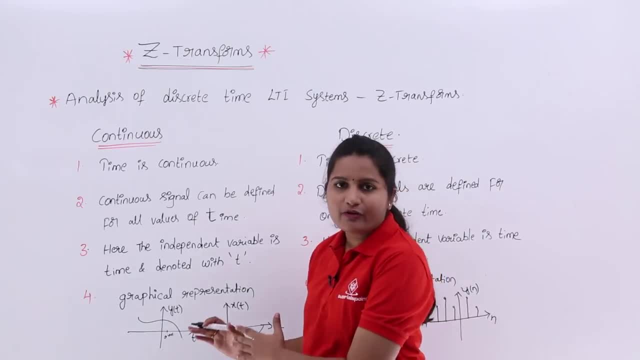 with n, The graphical representation of continuous time signal will be like this. Here you can observe, we can take function of t, for example. if this is y of t, y refers to name of the signal and y of t shows that it is a function of time. it is a continuous signal where t 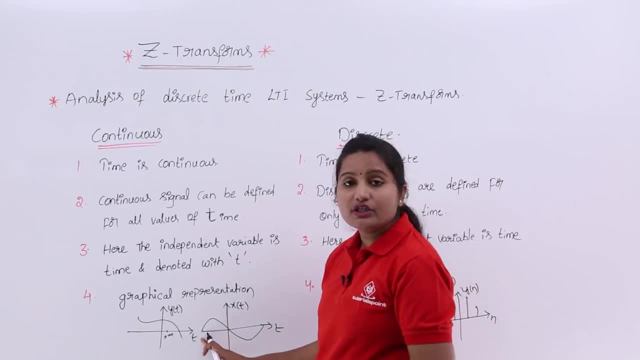 is a continuous time period. So in x axis you need to consider that time period. on y axis you need to note all amplitudes of x. You can also take any space or space into the general space over time. So in x axis you can consider that time period and in y 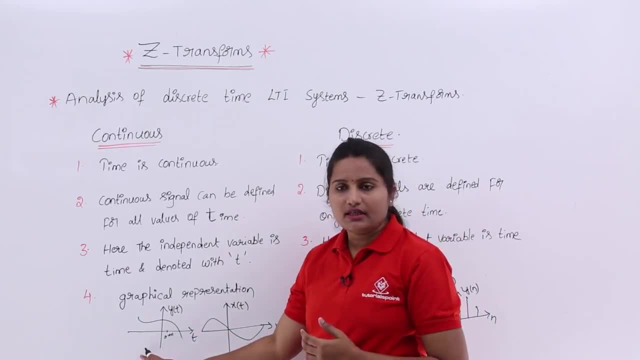 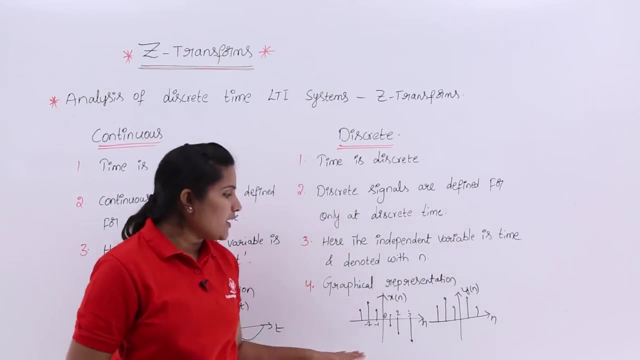 of the signals. as this is a continuous signal, you are having all amplitudes at all points of t. but here this is the graphical representation of discrete signal. here you cannot see the amplitude of the signal at continuous values. you can only see the amplitude of the signal at discrete values. 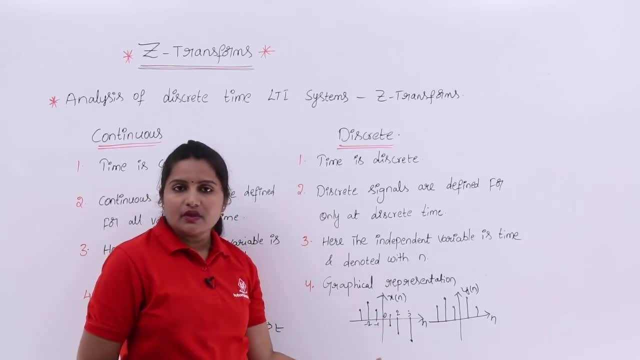 that means at 1, 2, 3, 4, only those are noted. and here also independent variable is time. but that independent variable time is indicated with small n. so here that small n will take on x axis and x of n refers to it is a signal with name x, x of n refers to that is a discrete.